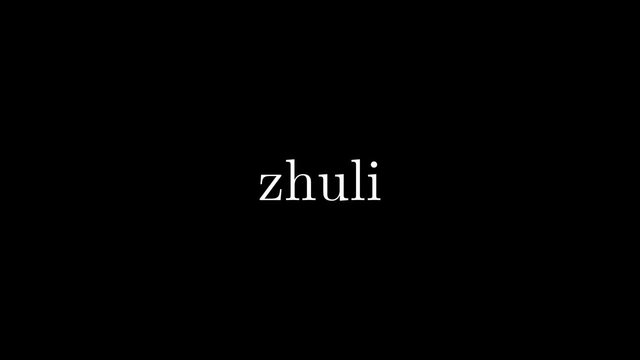 Here is a grid Starting from the top left corner, walking only along the grid lines in the right and down directions. how many ways can we reach the bottom right corner? Pause the video if you want to give this a try. The correct answer is 126.. Did you get it? 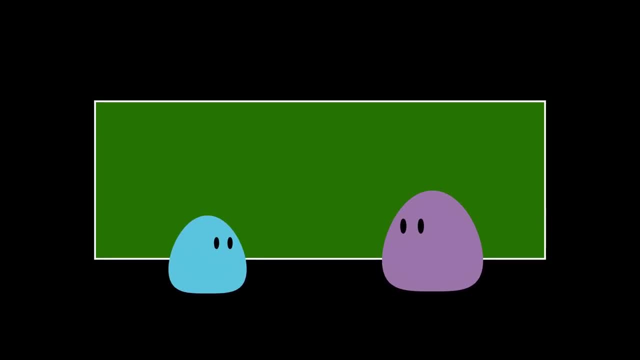 As I mentioned in the title, this problem changed my life. I remember when my teacher explained this problem to me in the seventh grade, and what I discovered and learned from the solution is one of the reasons why I love math so much today. I wanted to share that moment with all of you. 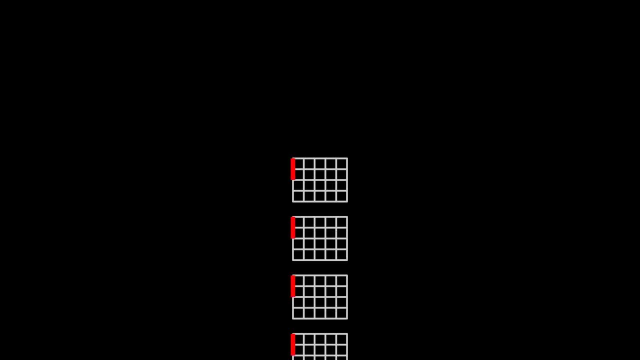 Let's first discuss how this problem is solved. The naive way to solve any counting problem is to make a list of all of the things we want to count and then just count the list. Clearly, this isn't very practical With 126 different paths. it would take forever to list them all. 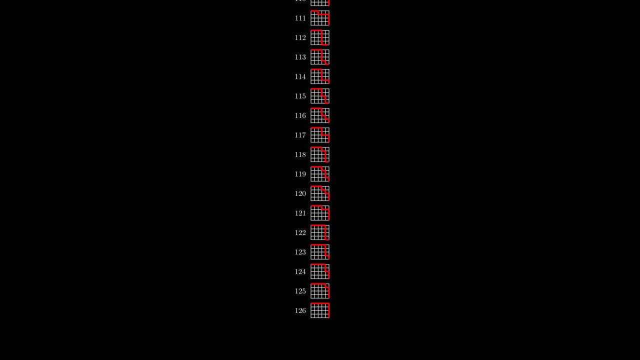 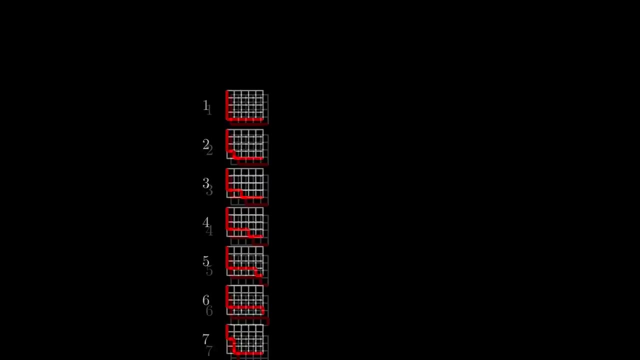 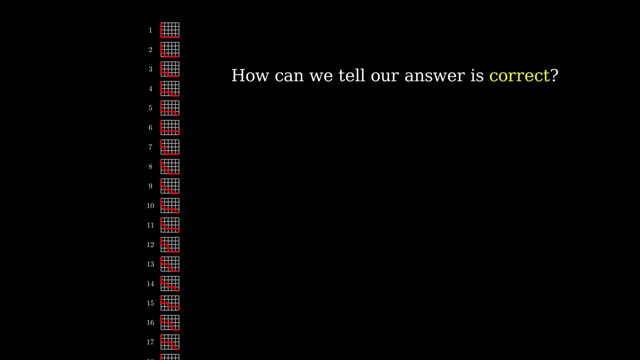 But, more importantly, because there are so many different paths to list, it can be very difficult to manage. I have the full list here, supposedly, but there are important unanswered questions. How can we tell that this answer is correct? How do we make sure that we haven't overcounted by counting a path more than once? 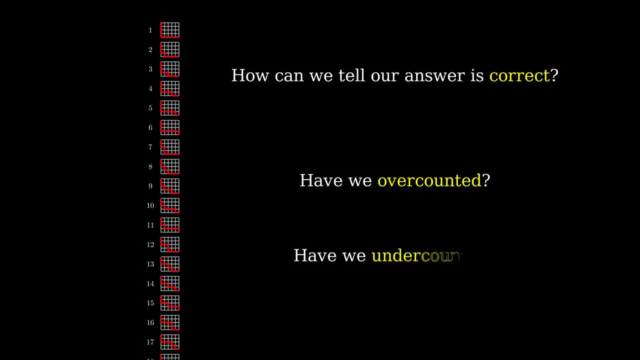 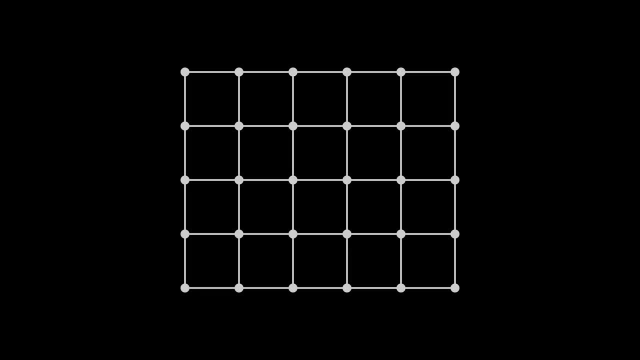 And how do we make sure that we haven't undercounted that there are paths that we missed in our list? Let's find another way to represent the path. Here is an example of a path I could take. How would you describe this path to someone? 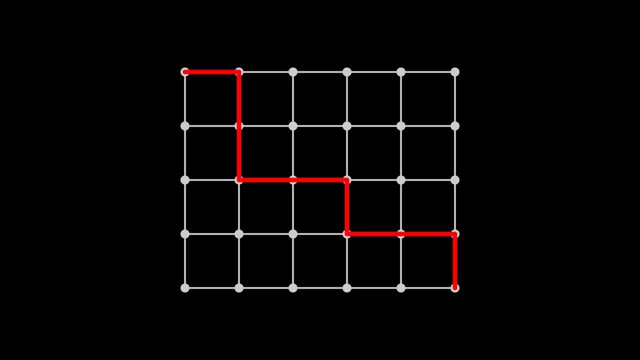 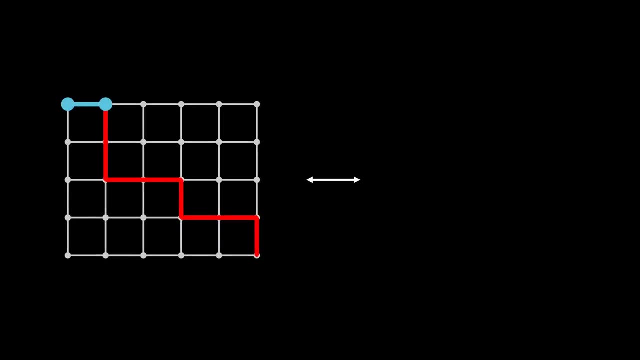 One way is to describe the direction of each step you take. For instance, here The first step takes us over to the right, so let's write an R to indicate that The next step goes downwards, so let's write a D to indicate that. 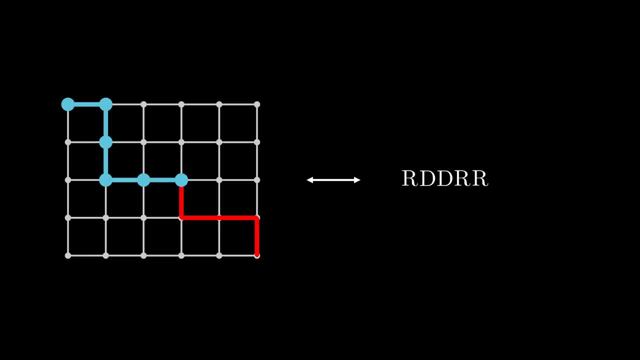 Continuing in this way, we make a sequence of letters that describe each step of our list. Notice that, using this method, there is only one way to describe the path and each sequence of letters can only produce one possible path. All we have to do now is take every single path and pair it with its step sequence. 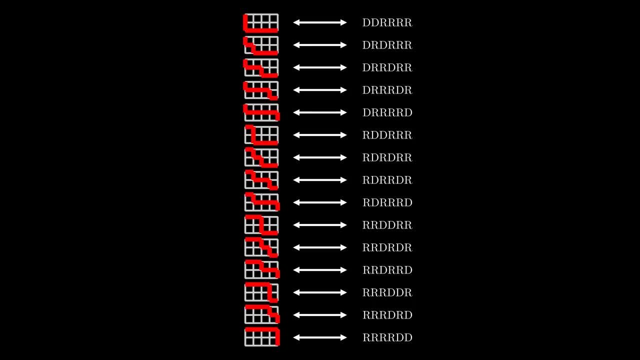 This example obviously isn't the same size as our original problem, but the concept is the same. The reason we are doing this is because both of these lists have the same number of things, So we can count either of these lists to get our final answer. 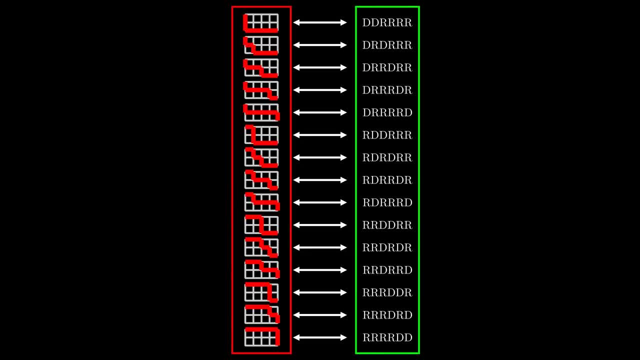 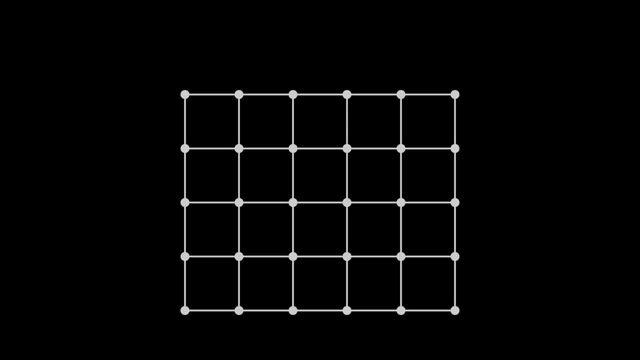 But the left list is much harder to count. The right list is much easier to count. Let's take a look at how we would count the right list. First of all, our path must contain 5 steps to the right and 4 steps downwards. 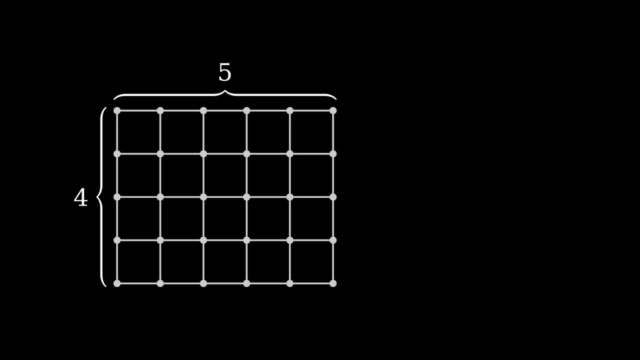 This means that our step sequence must contain 5 Rs and 4 Ds, for a total of 9 letters. Had the 9 letters all been different, the number of ways to order them is simply 9!. This is because there are 9 ways to choose the first letter, then 8 ways to choose the second letter, 7 ways to choose the third letter, and so on. 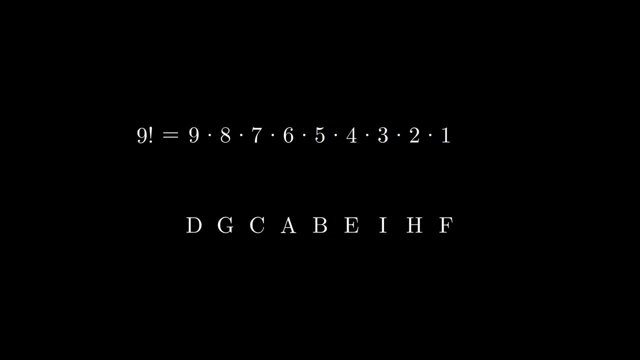 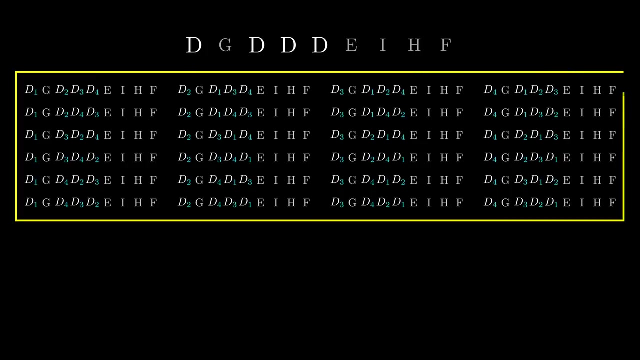 But there are 4 Ds. If we fix the other 5 letters, there are 4 factorial ways of ordering the Ds. Notice that we have counted all of these orderings, But they all should count as only one of the orderings we want, since the Ds are identical. 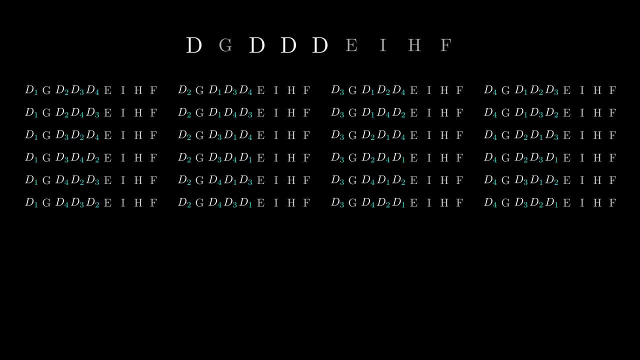 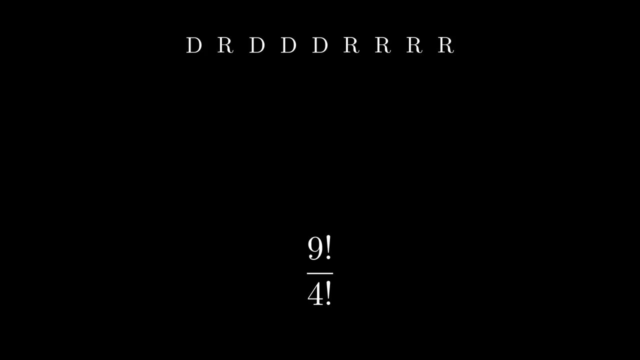 All of the orderings can be grouped in the same way, Which means that in order to account for the Ds all being the same, we need to divide 9 factorial by 4 factorial. Likewise, we can account for all of the other letters being Rs in the same way by dividing our account by 5 factorial. 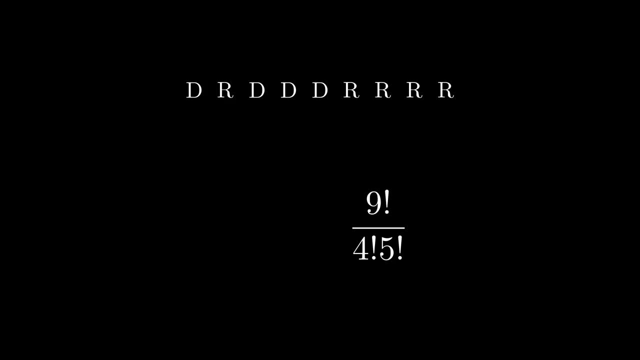 This expression gives us our answer. However, this is just the beginning. There is an established and simpler way to express this value. Another way to think about how we could make one of our step sequences is to simply choose any combination of 5 out of our 9 positions to make Rs. 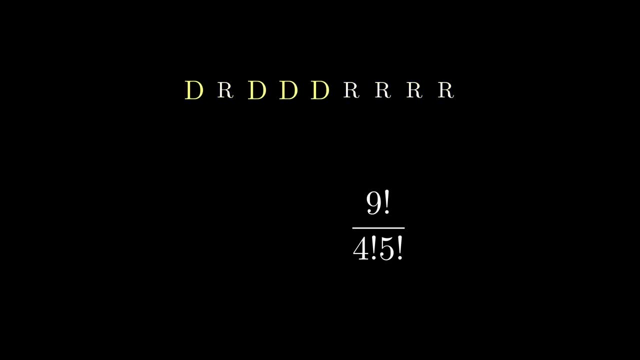 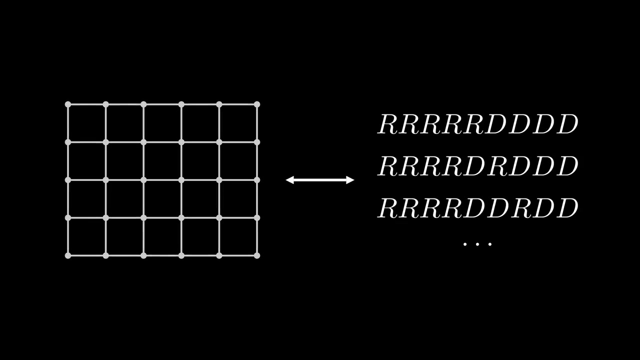 The rest will automatically be Ds. We call this value 9, choose 5, the number of combinations of 5 objects out of 9, written like this: So what did we learn? Well, for starters, notice that we started with a gridwalking problem, figured out an alternate way to list the paths, then figured out how to count combinations. 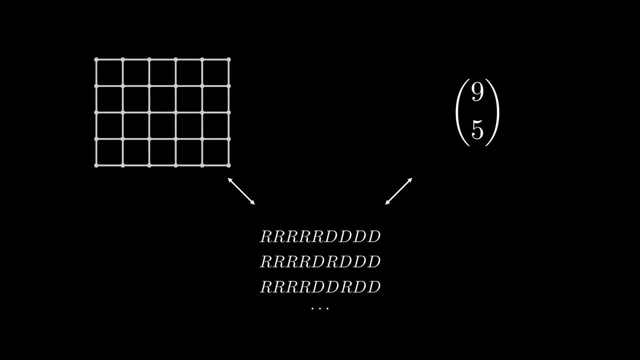 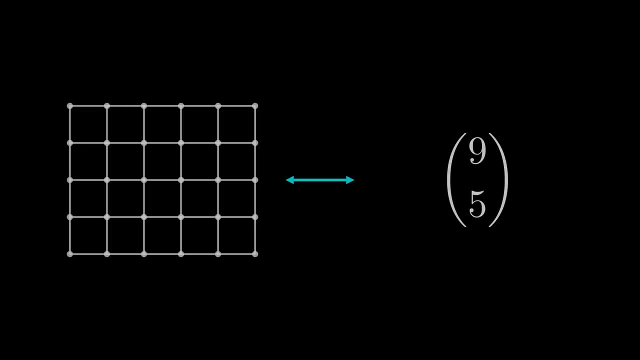 Thus the combination numbers are the solutions to our problem In general. for a grid that has x-width and y-height, our solution is: x plus y. choose x. This was the first spark of magic for me. Not only did this seemingly difficult problem have a very simple solution with an explicit formula. 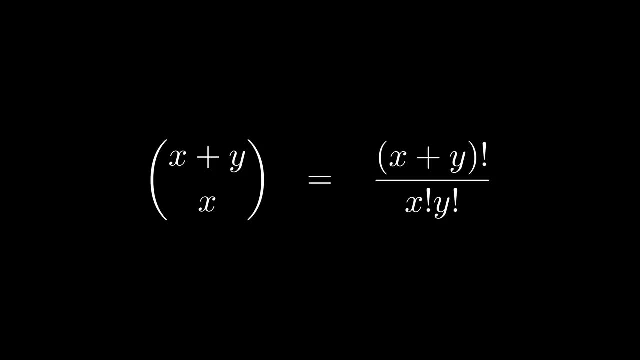 it was also the first time I saw a math problem that utilized a formula involving factorials. What's amazing, though, is that this isn't even the best part. It turns out there's another way to solve this problem, While there isn't an explicit formula. using this method, the concept is much simpler. 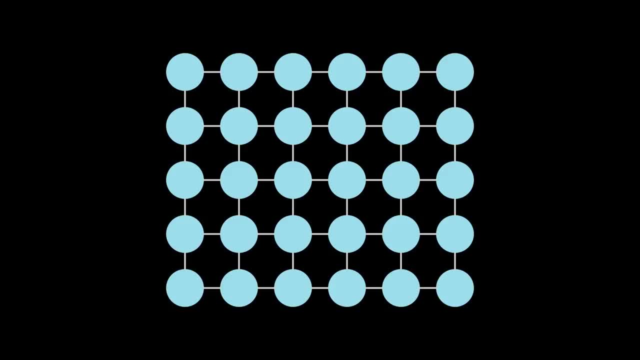 Let's label every point on this grid with a number, Specifically the number of ways of reaching that point. We start by labeling the starting point with a one. Some of you might be asking right now why we aren't labeling it with a zero. 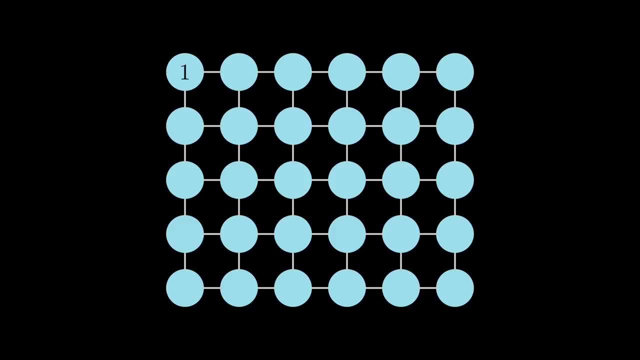 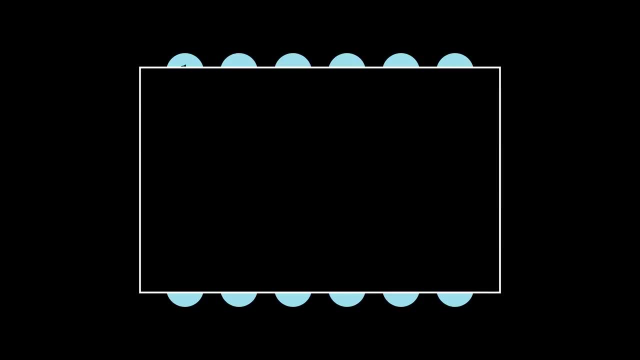 After all, if you need to end where you start, then you can't take any steps, so does that even count as a path? Well, think about what it means to say there are zero ways to reach somewhere. If I say that there are zero ways to get from point A to point B, I'm basically saying that it is impossible to get from A to B. 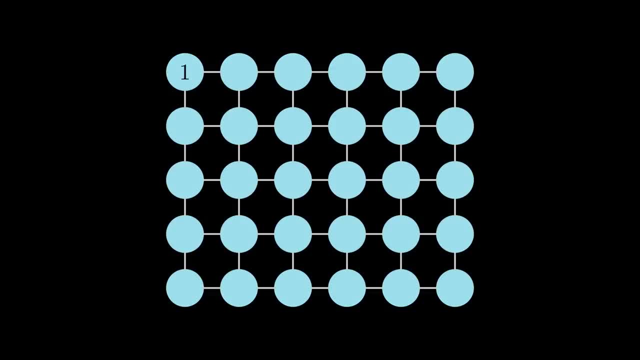 Clearly, it's not impossible to reach my starting point, since I'm already there, And so we want to say that there is exactly one way to get there. Next, notice that all of the points directly to the right and down can only be reached in one way. 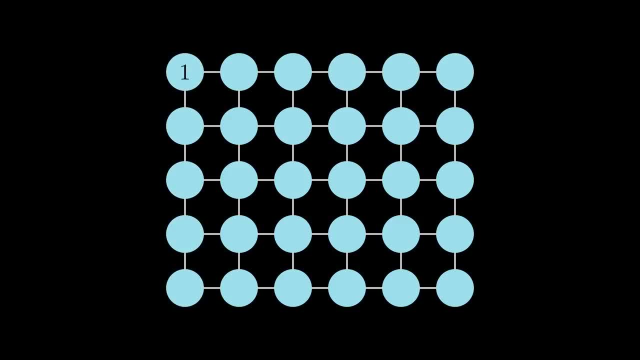 And so we can label all of these points with a one. This point here is a two, since there are clearly two ways to get there. However, there is a more general logic. Notice that there are only two ways we can approach this point. 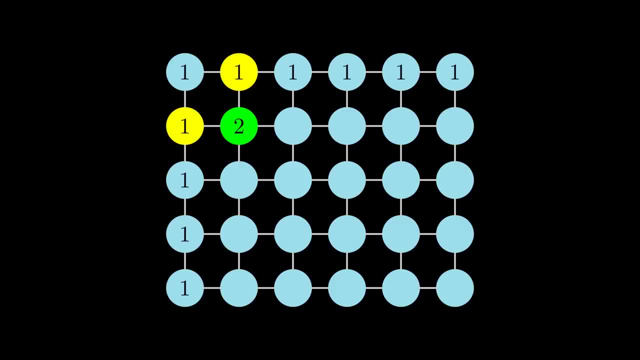 We either approach from the left side or the top side. Therefore, the number of ways of getting to this point is the number of ways to reach the left point plus the number of ways to reach the top point. All we need to do is add these numbers and we can find the number of paths to get here. 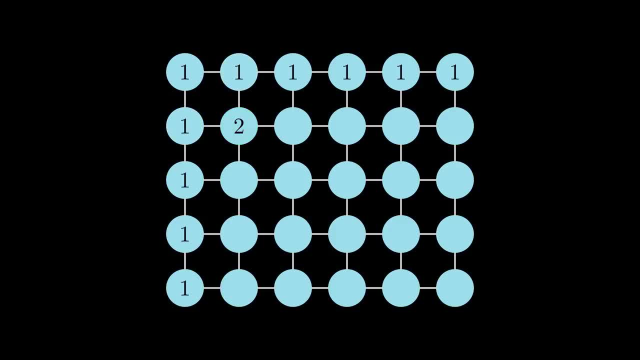 We continue this approach And fill in the numbers, eventually reaching the bottom corner where we get our answer Pretty slick right. Well, don't go yet, because I saved the best for last. There's an amazing and important reason why I showed you both methods. 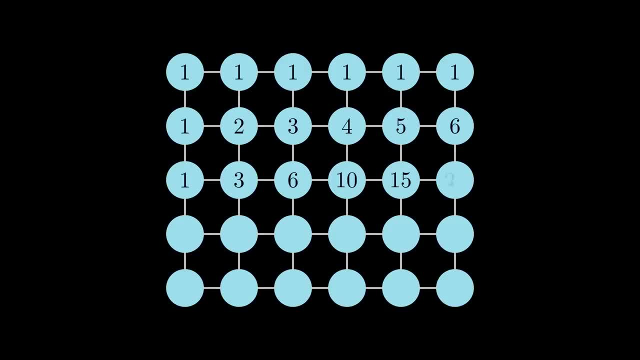 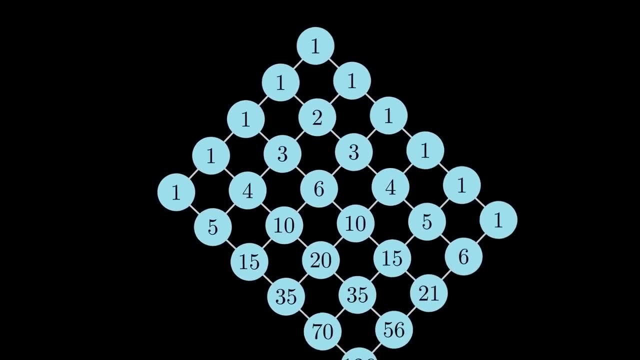 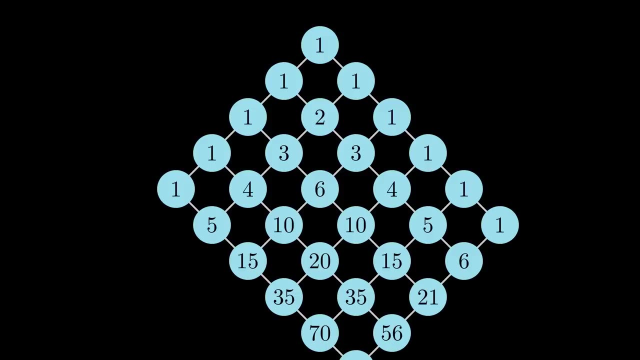 So let's label all of the points like we did before. I'm going to do something kind of subtle to the grid now And there I've rotated the grid about 45 degrees. Now, some of you may recognize this, but for those of you who didn't, this is a part of Pascal's triangle. 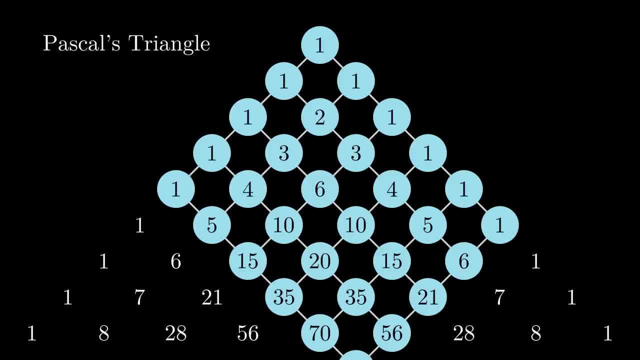 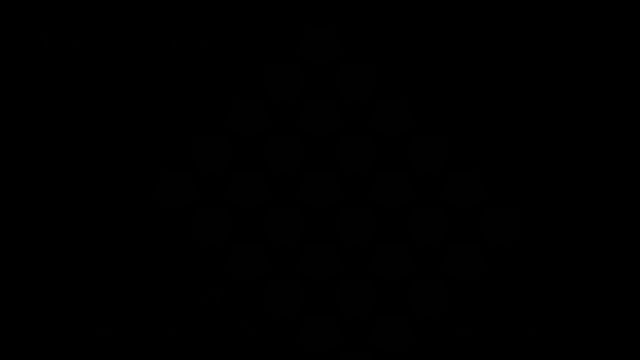 Pascal's triangle is the pattern you get when you start with a one at the top. then make each number underneath the sum of the two numbers directly above it. Okay, Let's reset for a minute. So let's label all of our points like we did before. 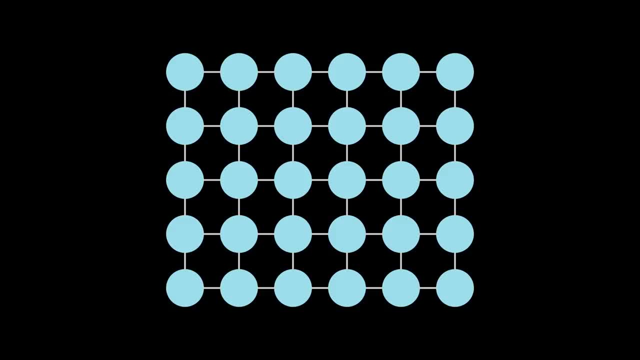 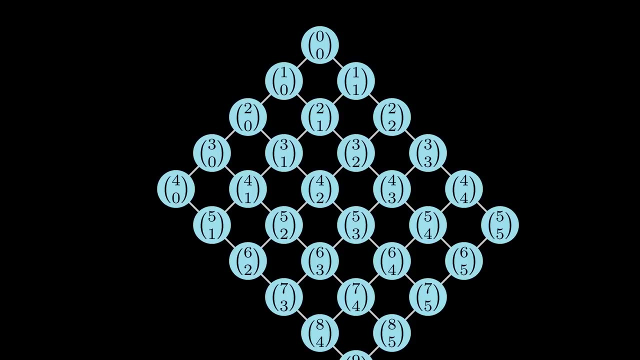 Except this time, instead of writing the counts as numbers, let's use the formula we figured out, Since it's the same problem. the values are the same. What this tells us is that Pascal's triangle is essentially a table of our combination numbers.